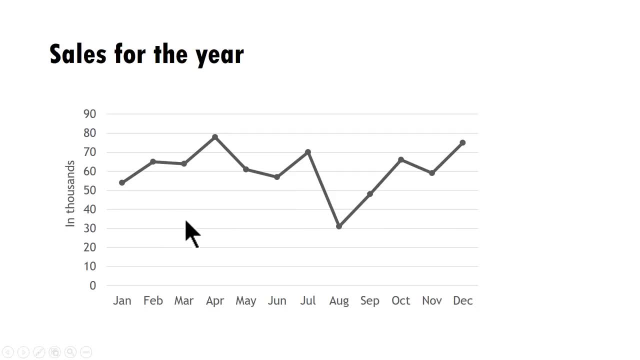 shown here. The reason why line chart works so beautifully to show trend over time is you have these various data points and it connects those various data points visually so your eye can follow the trend, and that is the reason why it is always advisable to show a trend using 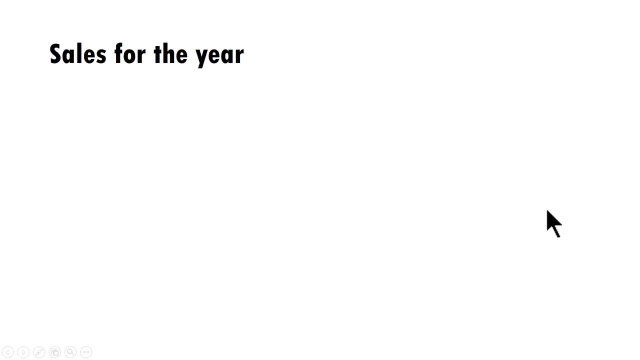 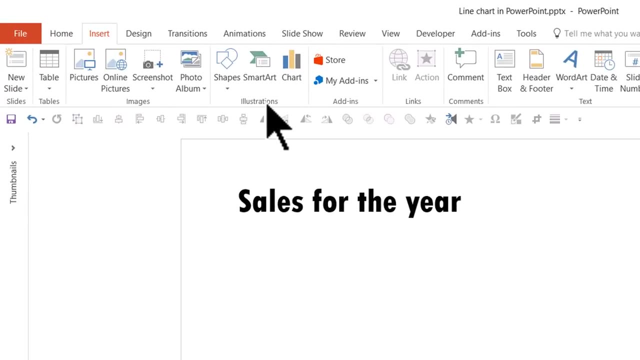 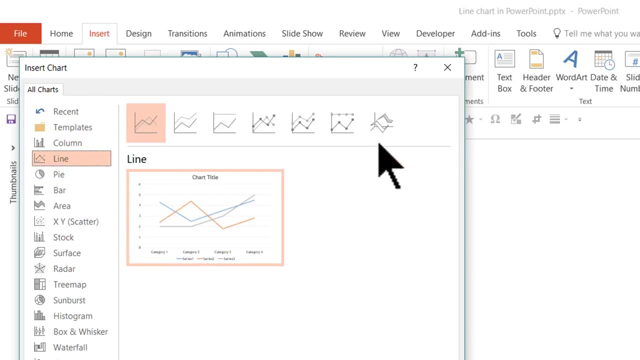 line chart. To create a line chart, all we need to do is go to a new slide. Let me go to insert, and here in illustrations group you have chart. The chart type we would like to use is line chart, and here you can see that there are a whole bunch of options for line charts. The one that I prefer to use is 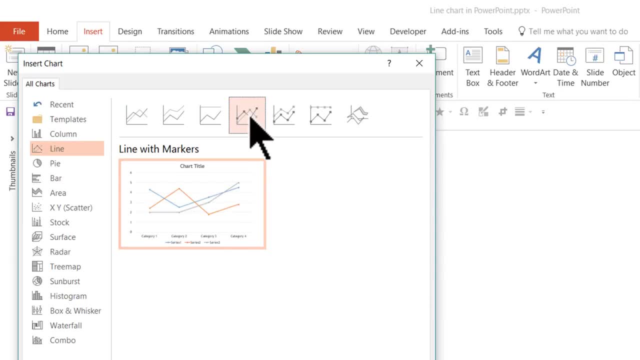 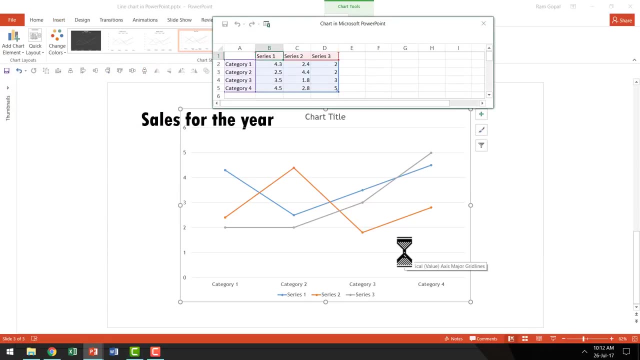 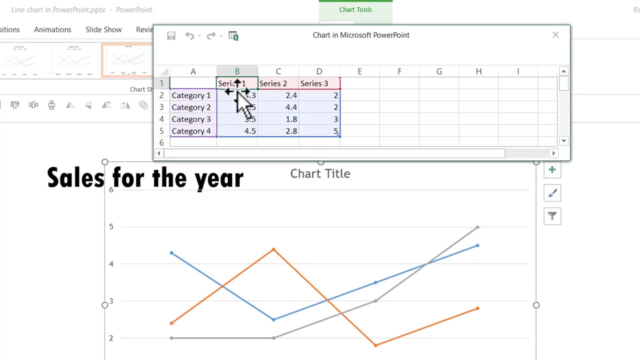 this one called as line with markers. It is a simple stacked line chart with markers. I am going to say OK, And that inserts the line chart onto my slide. Now you can see that there is an accompanying worksheet that gets opened simultaneously and we can replace the sample data with our own data. 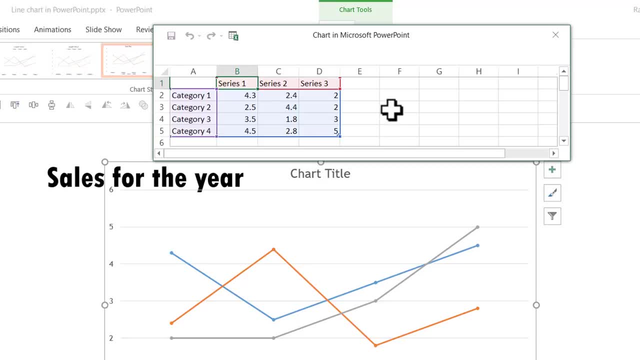 In this case, I am going to use the sales performance for just one year, So I need one series and I don't need all these additional series which are shown by different lines here. I am going to click and select all these two lines here. 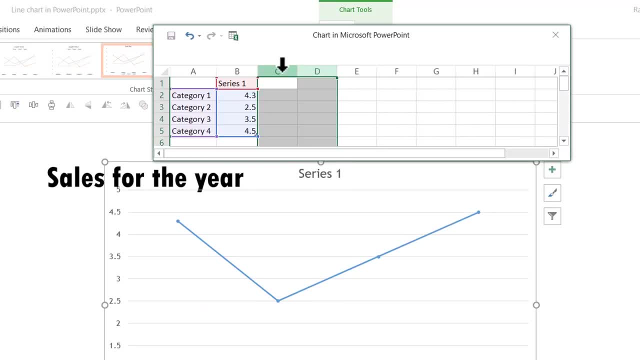 I am going to right click and say delete, and that deletes those other unnecessary series here. As you can see here, to select an entire column all you need to do is to place your cursor on the header and then click, and then you will see that the entire column gets selected. So that is the way that we. 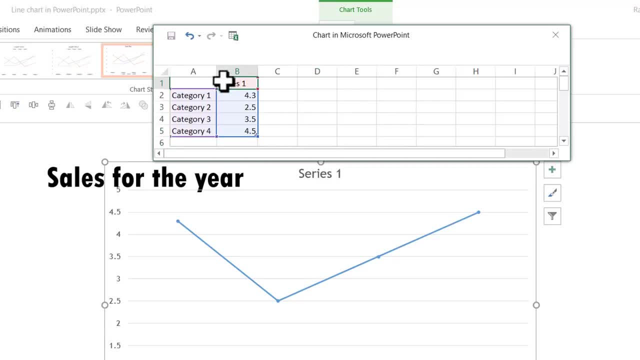 select the column and delete. Now I am going to replace this series one as sales, and then we are going to replace the categories with months. I am going to make some space Because want more than just four values here. I want to add more, So I am going to click and drag this. 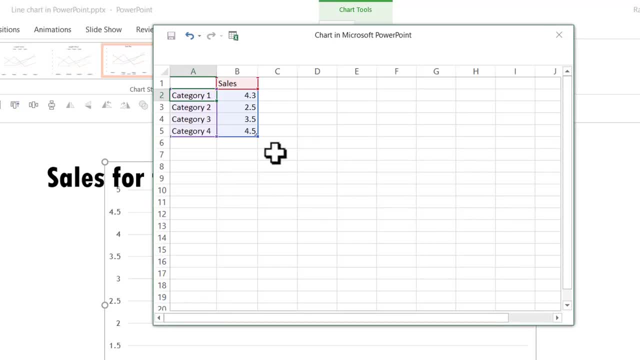 down. So that is another thing that you may want to know, and that is, you can always expand this worksheet to suit your requirement. The next thing is: I am going to enter my value here, So I have written Jan and, as you can see, there is this cross that comes when I move my cursor to the bottom. 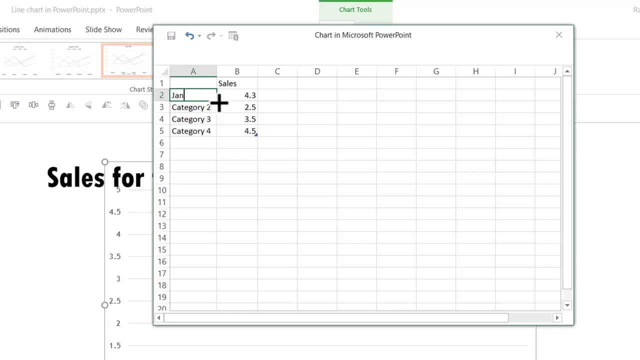 right corner and that is my shortcut: to add more months without having to type them all. So I am going to click and drag across and you can see that I can drag beyond the highlighted portion and as I move my cursor down you can see that each additional month is getting added, The last month, 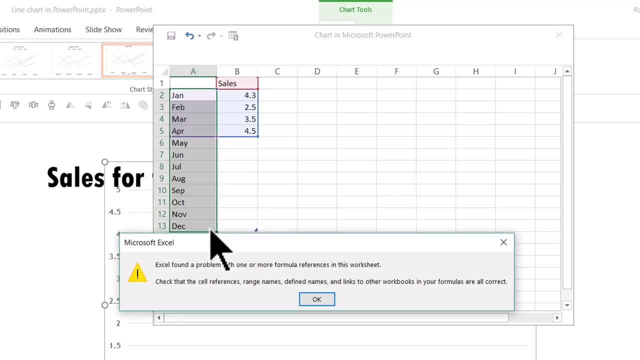 is December and I can release my mouse, click and immediately all the months are populated. Now this says: Excel found a problem with one or more formula references in this worksheet and I have not really added any formula, So I am just going to say: okay, you, it is important for you to read all this stuff before you take action In this. 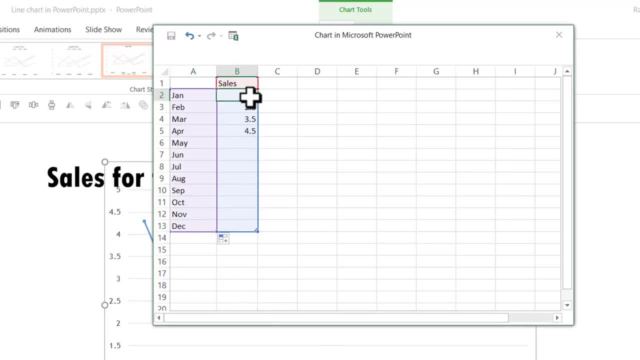 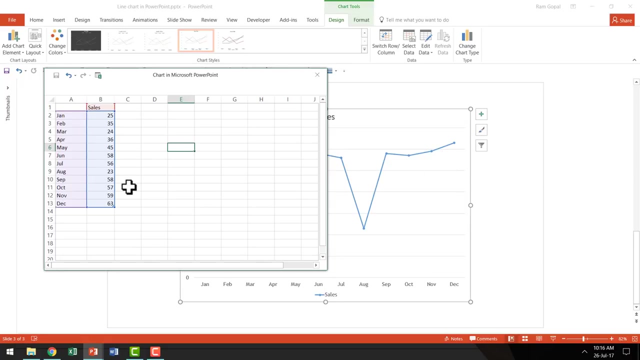 case, I am just going to say okay and then I am going to add my numbers here and I am going to enter random numbers. So let us pretend that these are the performance values for the various months here. and as I move my worksheet you can see that there is a beautiful line chart. that is already. 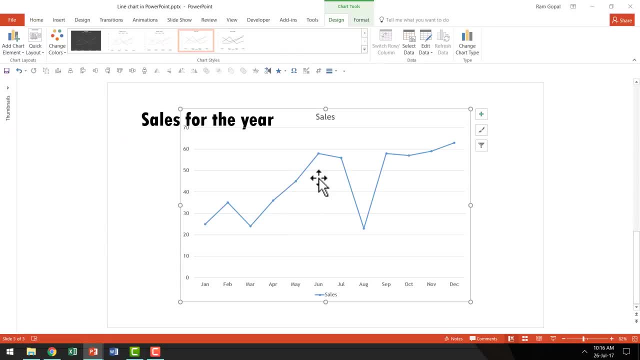 created, and I am going to just close this. When I go here, you can see that I have a beautiful line chart ready. I can always click and drag this white circle here to resize my chart. Now there are so many things you can do to make this chart better. One of the things is: 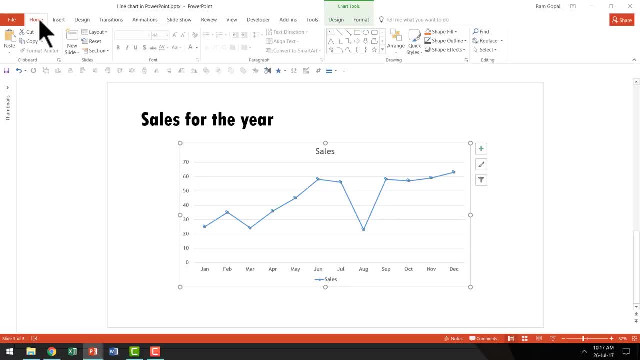 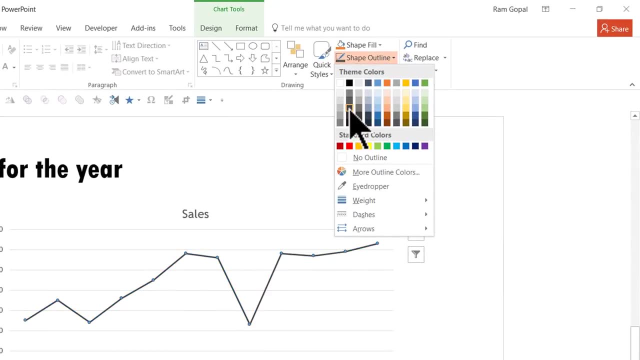 you can click on the line and you can go to the Home tab. in PowerPoint ribbon, go to the shape outline and you can change the color of the line. I prefer to use black color because it's a very neat and and visible color and if I want, I can always go here and increase the weight of the line, just as. 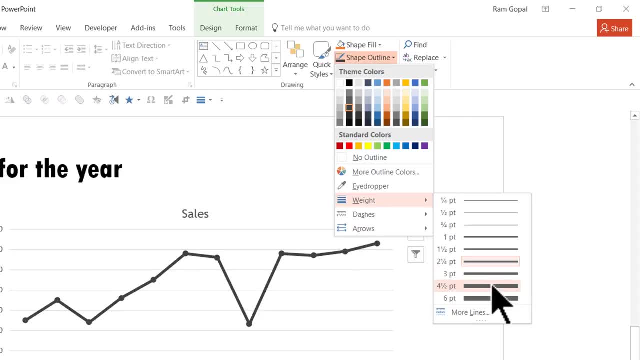 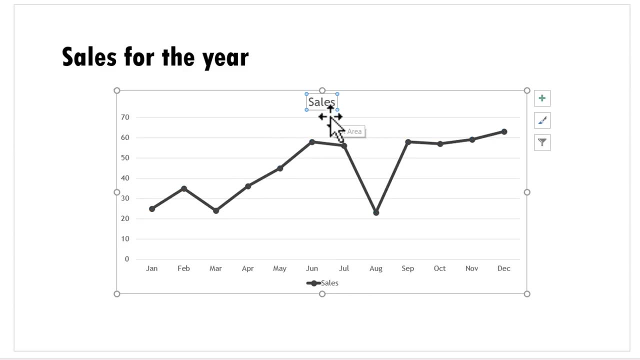 you would do with any line, and I prefer to have the line slightly thicker, so around four and a half points. and another one that I do is if there is only one data series, there is no point in having these legends, and therefore I'm going to click here and delete. Another thing that I do is I 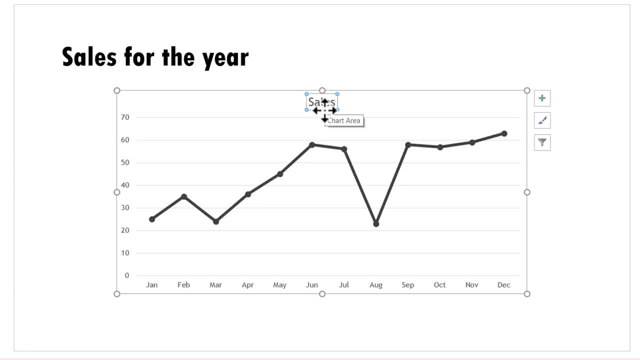 always prefer not to have any chart title, because my chart title is going to be my slide title, so I'm going to select this and I'm going to delete it. Now this looks much cleaner. The one last thing that I need to do is to make sure that these fonts are a lot more readable, so I'm going to click.